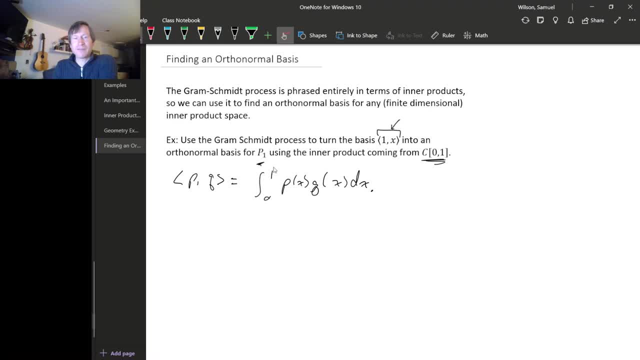 And exactly the same thing is true of any other inner product space. So you can imagine if you were going to do a bunch of projection calculations in P1, you'd really like to have an orthonormal basis. So let's work out an orthonormal basis. 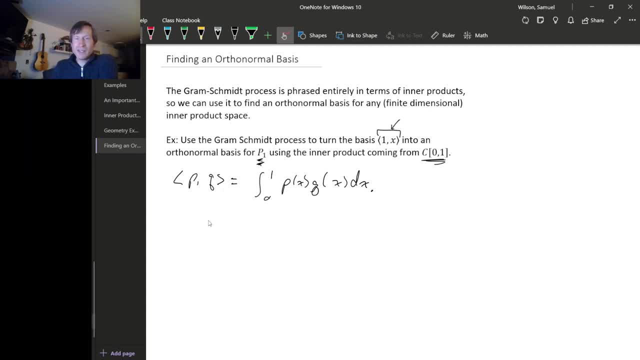 So to do Gram-Schmidt, remember what we need to do is So the first ELF element in the basis you leave alone, right? And then the actually? well, yeah, there's more than one way to do Gram-Schmidt. The general idea is always the same: you just take your vector and subtract off projections onto earlier basis vectors. but the details of like when you normalize things depends on who you're talking to. 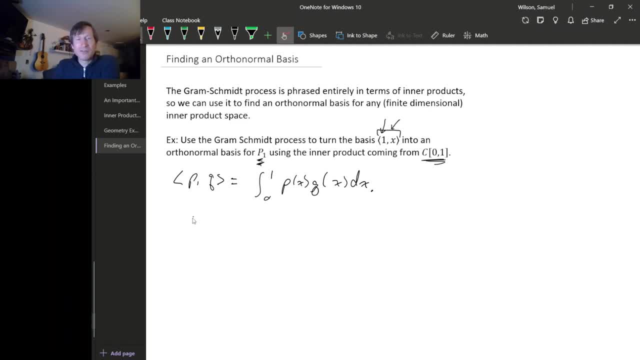 Um, fortunately we don't need to worry about when to normalize this first basis element 1, because its norm is actually 1,. so right, if we just calculate the inner product of 1 with itself, that's the integral from 0 to 1 of 1 times 1, but that's 1.. 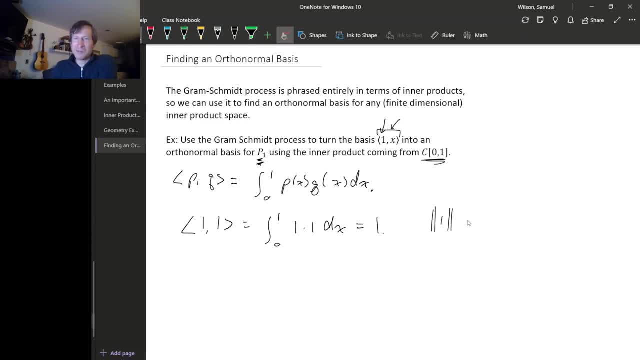 So the norm of the basis element 1 is 1.. In other words, 1 is already a unit vector. Okay, so for our second basis element. so I guess that's going to be our first basis element, the polynomial 1.. 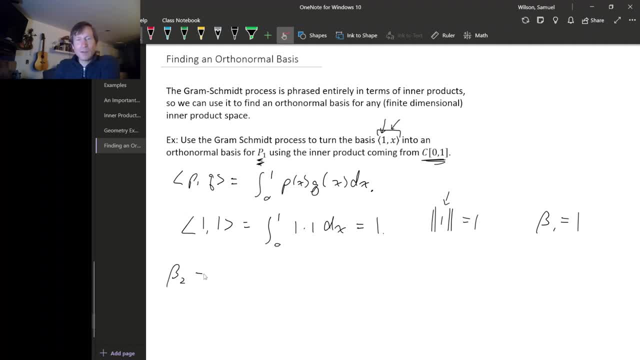 So for our second basis element, we take, for our second basis element, for the orthonormal basis that we're producing, we take our second basis element for the basis that we started with and then subtract off the projection onto the basis. 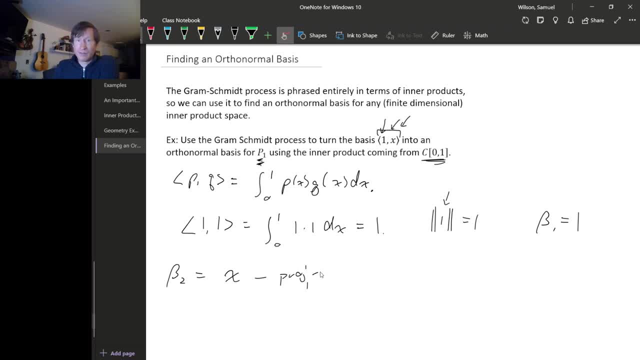 So that's going to be our second basis element, and then subtract off the projection onto the first basis element of our second basis element, right, So right, this is exactly the same formula as Gram-Schmidt in Rn, right. 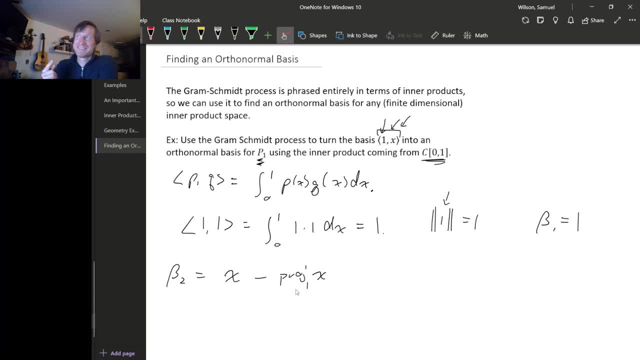 It's just that our vectors aren't vectors in Rn, they're polynomials of degree less than or equal to 1.. Okay, so this is x minus. so what is this projection? Well, again, the formula for a projection is exactly the same. 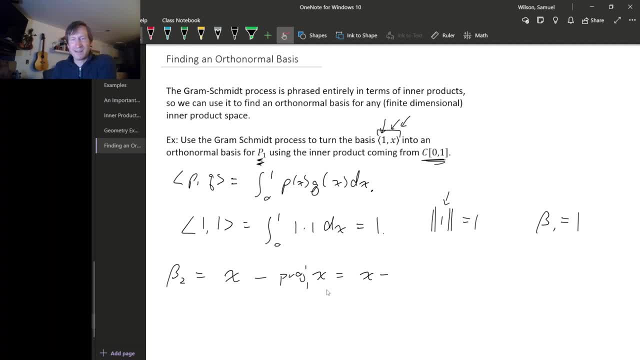 in an inner product space, as it is in, as it is in Rn. So it's the inner product of x and 1 divided by the magnitude of, or the norm of, 1 times the vector 1.. Of course, we know that the norm of 1 is 1, so we don't need to calculate this again. 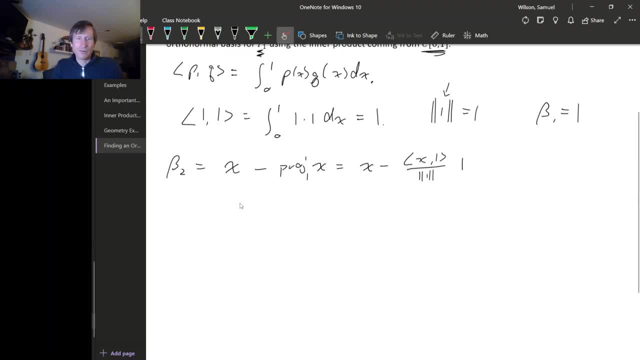 But we need, we're going to need to calculate this inner product of x with 1.. So that's inner product of x with 1 is the integral from 0 to 1 of x times 1,. so that's right: 1 half x squared from 0 to 1, that's a half, okay. 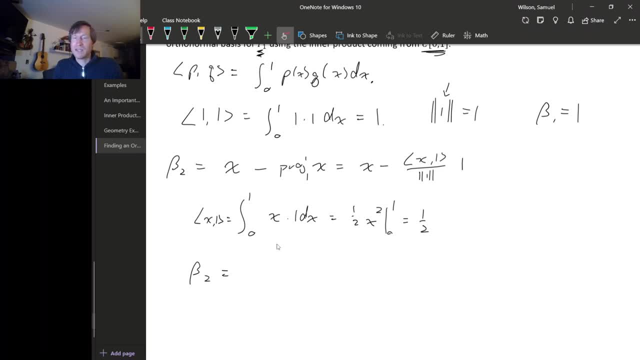 So this beta 2 that we're calculating is x minus right. this right here we now know, is a half. so x minus 1, half right. this is the scalar 1 half times the polynomial 1, but that's the polynomial 1.. 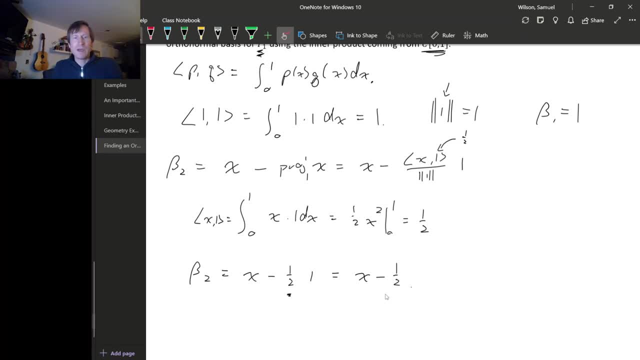 The polynomial x minus 1 half. okay, Now we need to. so this: remember when you do this calculation in Gram-Schmidt, the result might not be a unit vector. It definitely is orthogonal to the previous vectors in your basis. 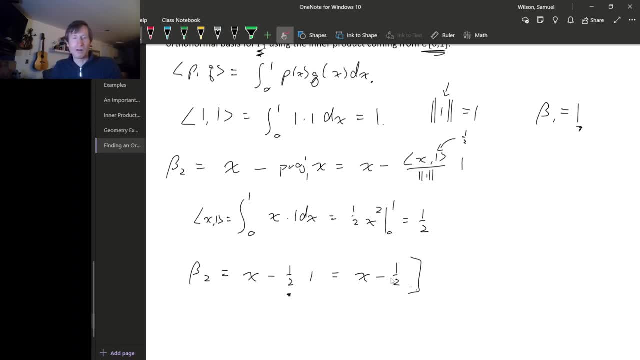 We won't. I won't check that, but it is. these two are orthogonal. But this vector might not be unit length, so we need to calculate its norm. So we need to calculate its norm. So x minus 1 half and x minus 1 half, so this is integral from 0 to 1. 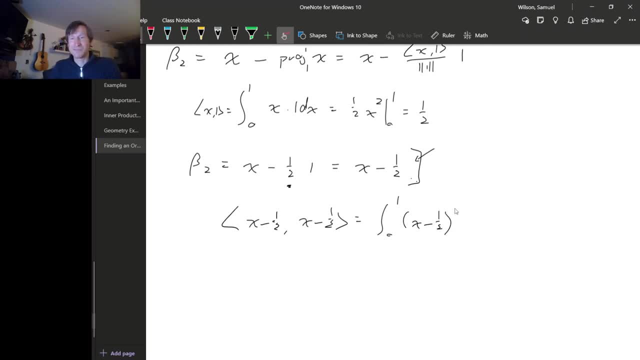 of x minus 1 half times x minus 1 half, so that's x minus 1 half squared dx. So this is integral from 0 to 1 of x squared minus x plus 1 quarter, I guess. So this is 1 third x cubed minus x minus 1 half. okay. 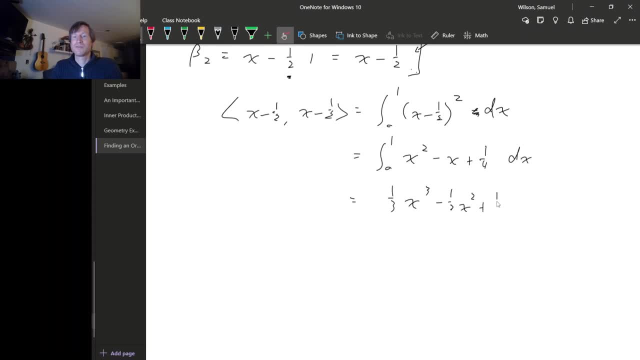 So this is 1 third x cubed minus 1 half x squared plus 1 over 4x, and we need to evaluate at 0 and 1, and so we get a third minus a half plus a quarter. So a third minus a quarter, that's a twelfth, I think, right.